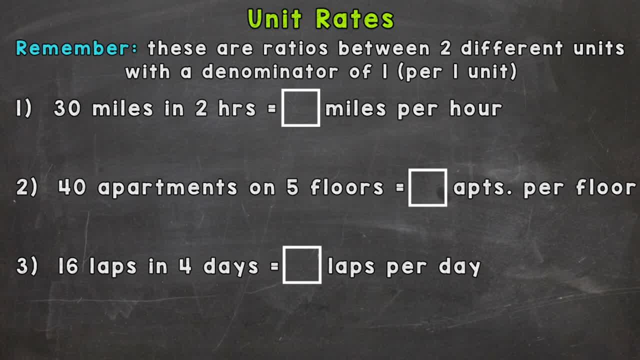 That might not make complete sense right now, but as we go through the three examples on your screen, you'll start to see what I mean by the per one unit. So let's jump right into number one, where we have 30 miles in two hours. 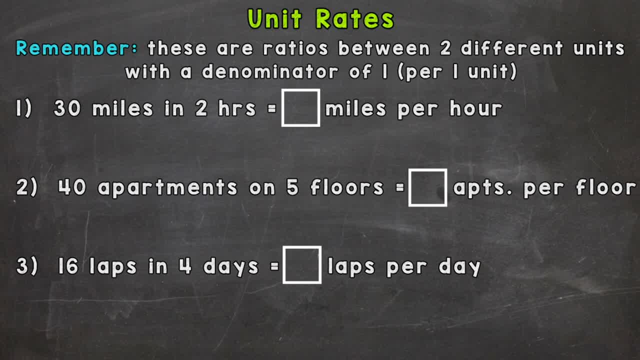 We need to find how many miles there are per one hour. So we find a unit rate by writing out our ratio as a fraction. So we have 30 miles per two hours. So I'll put miles hours here. So what we need to do, we need to get a denominator of one. 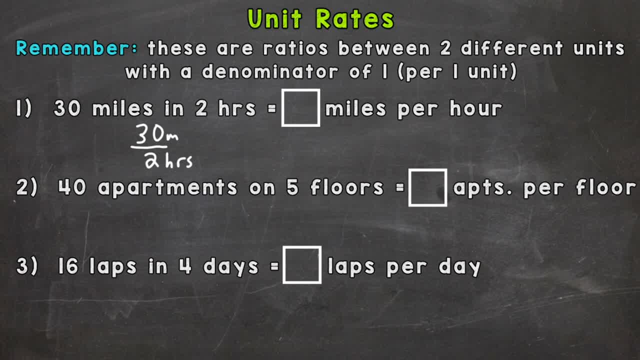 That's going to give us per one hour here. So, in order to get a denominator of one, how do we get that two to equal one? Well, let's divide it by two, And with fractions, in order to keep that equivalent. 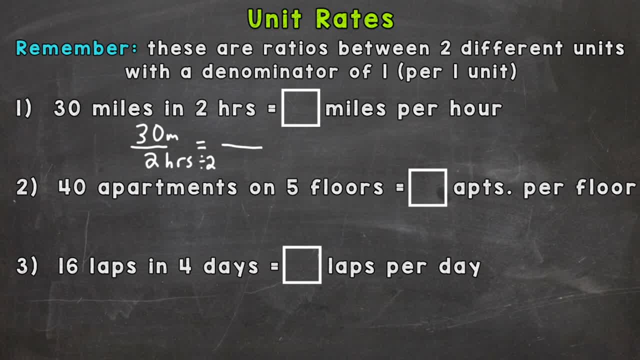 so we don't change the value. whatever we do to the bottom, we must do to the top. So we need to divide The 30 by two. that will keep everything equivalent and give us the unit rate, because we'll have a denominator of one. now. 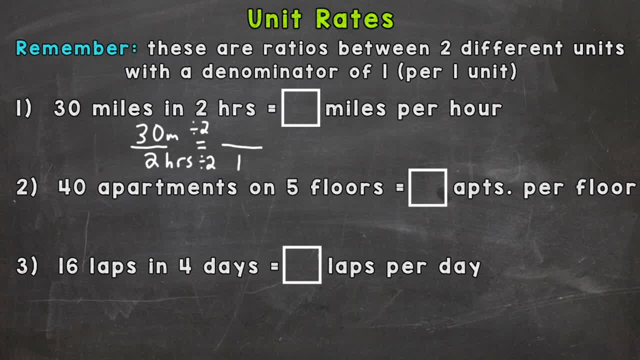 Two divided by two is one, 30 divided by two is 15.. So now we have 15 miles per one hour, or 15 miles per hour. So 30 miles in two hours equals 15 miles per hour. So that's our unit rate. 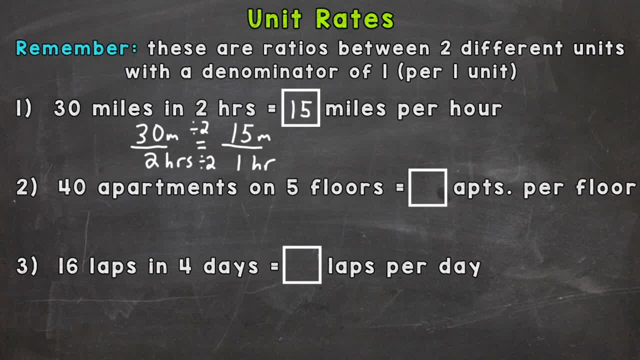 Number two: 40 apartments on five floors, So we want to find how many apartments per floor. So again, let's set it up as a fraction: 40 apartments on five floors, So we need to find out how many apartments per one floor.